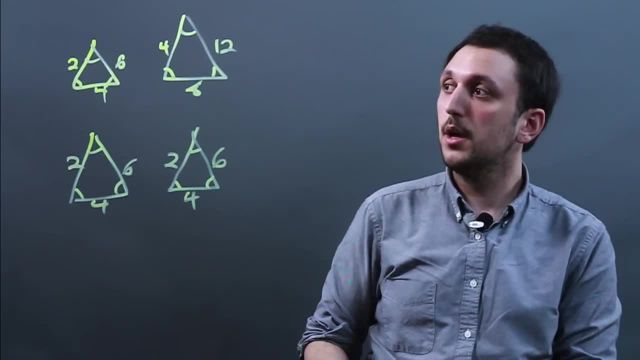 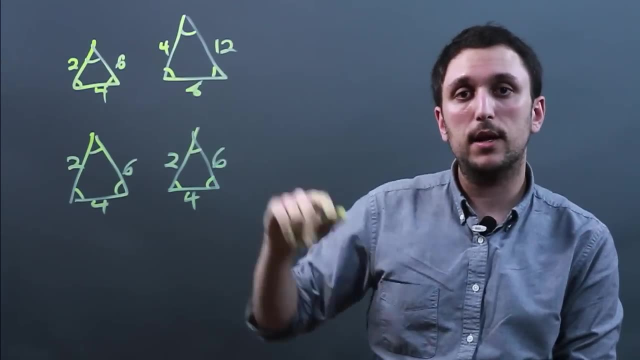 6. So you've just learned the difference between congruent triangles and similar triangles. Congruent triangles have to be exactly the same. Similar triangles just have to have the same angles. I'm Charlie Kasov. Thanks a lot. 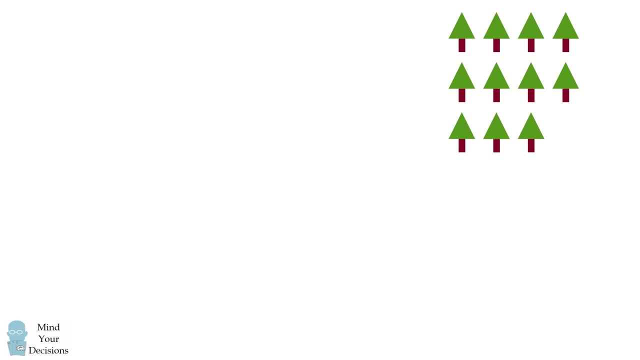 Hi, this is Presh Talwalkar. This riddle is a logic puzzle and it assumes that the characters can reason with absolute precision. so pay attention to the details of the story. Alice and Bob are trapped by an evil logician In their cells. Alice can see exactly 12 trees. 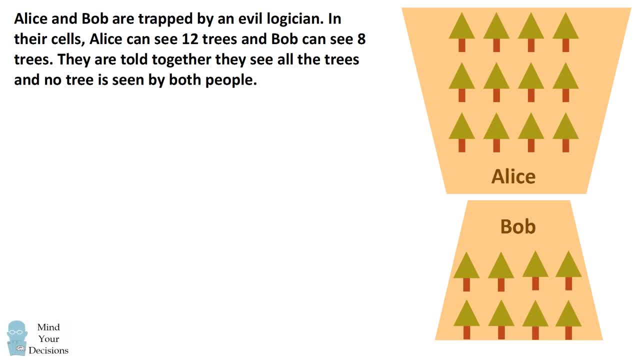 and Bob can see exactly 8 trees. They're told that together they can see all the trees in the prison, but that no tree is seen by both people. Neither person knows how many trees the other person sees Every day. the logician visits Alice in her cell in the morning and asks: 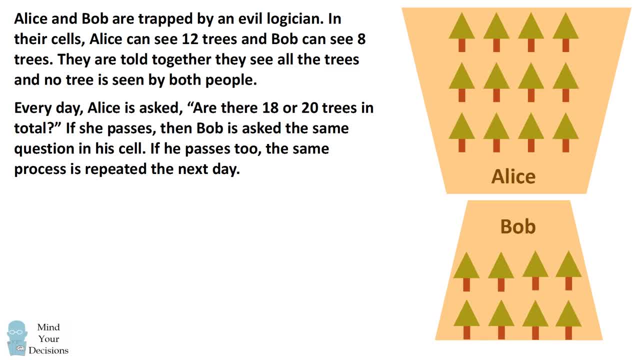 are there 18 or 20 trees in total? If Alice knows the answer, she can say, but if she doesn't know, then she's going to pass. In that case, the logician then goes, visits Bob in his cell and then asks the same question. If Bob knows, he can give the answer. otherwise 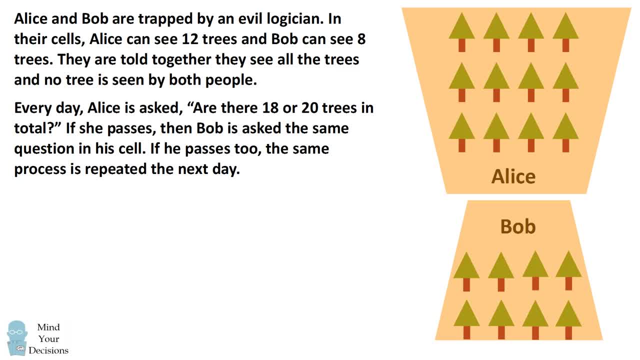 he also is going to pass. If they both pass, then the same process is repeated the next day. The logician then goes to the prison to investigate. Now, at some point they're going to want to guess, because they don't want to keep passing. 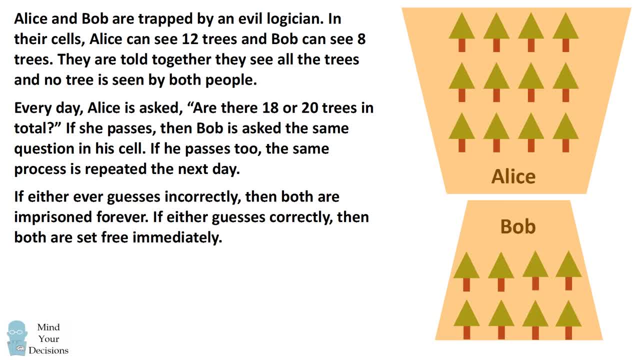 and staying in prison forever. However, if either person doesn't know and they guess incorrectly, then they're both going to be imprisoned forever. If either person does know and guesses correctly, then they're both going to be set free immediately. Now they can't communicate with each other the number of trees that they see. 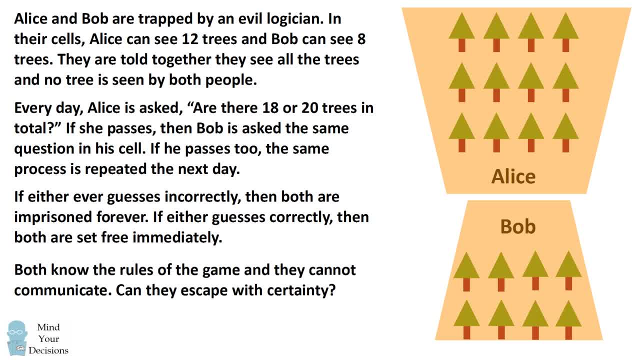 but the question is: can they do better than random chance? Can they do better than just guessing 18?, 18 or 20.. If they both understand the rules of the game, can they escape and reason their way out with certainty. Give this problem a try and when you're ready, keep watching.